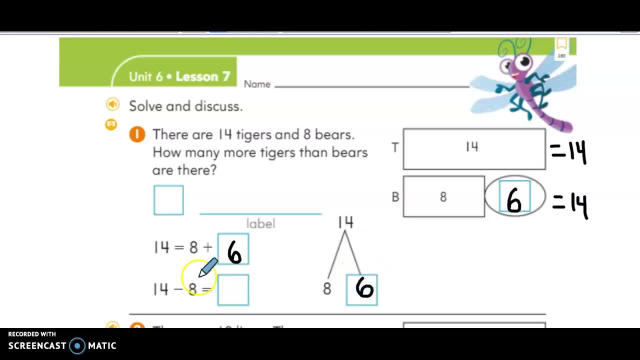 It's only sort of missing out once you've done that choice 11 and 8.. How do we kinda trick them? Well, there are some ways to do Promise D: You can work with your partner together to give us 14.. Okay, Lastly, we have the subtraction problem, which we can also use subtraction to figure out these problems: 14 take away 8, so that would look like if you were starting on a number line. you would start at 14 and take 8, hops backwards. or you could start at 8 and count up to 14 to find what the difference is between those. or, if you want, you could even say the number 14 and count backwards. 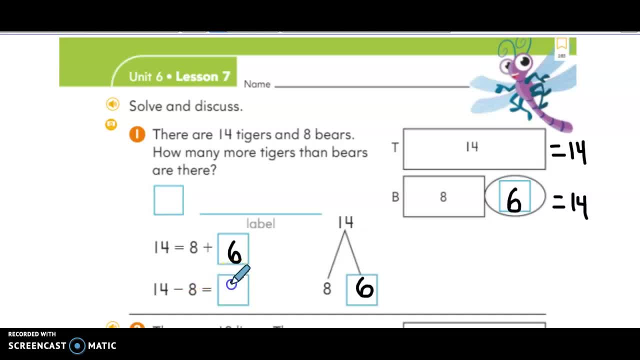 putting up a finger with eight fingers. Either way I'm going to come up with six. So all these unknown boxes are going to match And we have to check our question for the label. Our question says how many more tigers? So if it's in the question, we need to put it in the label: more. 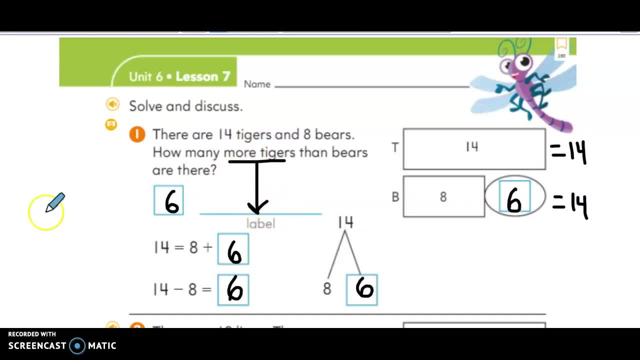 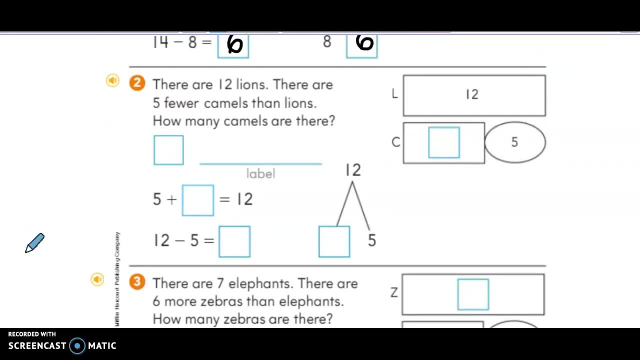 tigers. So you're going to write that: more tigers. Okay, let's do number two. There are 12 lions. There are five fewer camels than lions. How many camels are there? Okay, notice that they labeled the lions at the top, because there's more of them. 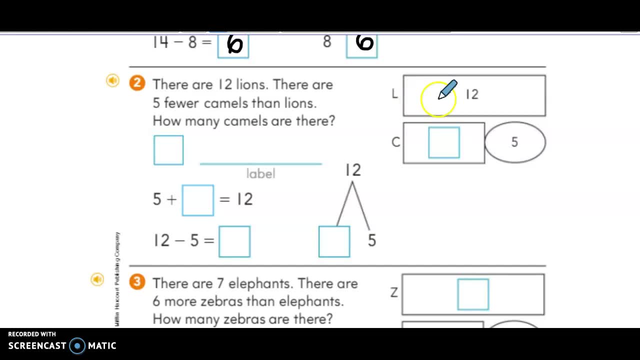 right, We're always going to put the one that has more on the top, And there was 12.. Then the next thing it told us is that there are five fewer camels. Okay, they put camels here. Five is with the word fewer. We know when we hear that word we're going to put the word fewer. So we're going. 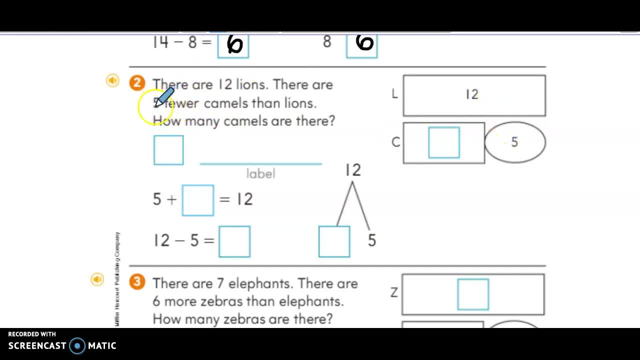 ding, ding, ding. It goes into the oval. Okay, five fewer means that's the difference. It goes in the oval. So we're looking for the actual amount of camels that there are. Okay, let's put our equal signs out here: Equals 12,, equals 12.. Okay, so we have unknown. plus five equals 12,. 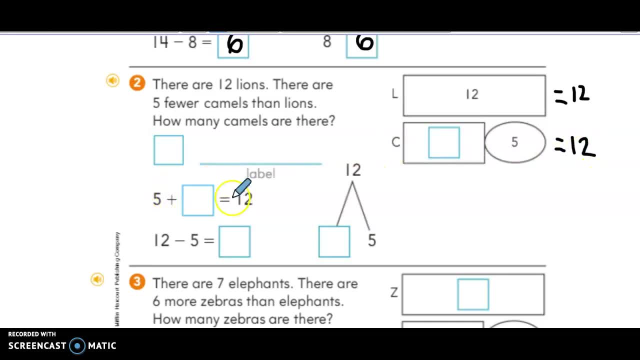 as you can see right here. Okay, they just switched it around a little bit, and that's okay. And then we have our math mountain: Five partners with what to get us 12?? We also have another option: 12, take away five, equals what? Okay, see, if you can figure that out. 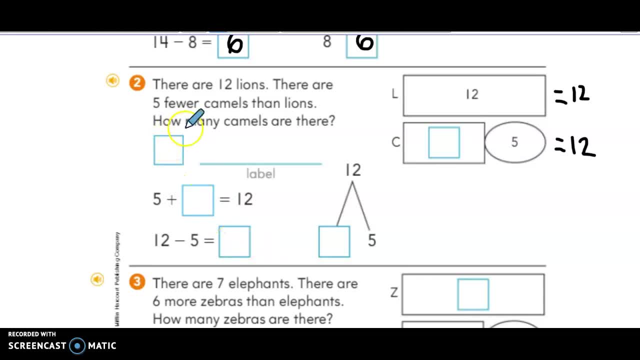 All the unknown boxes will be the same. Check your question for the label. How many camels are there? Well, it doesn't have any special words attached to it, so it's just going to be camels. Okay, number three. 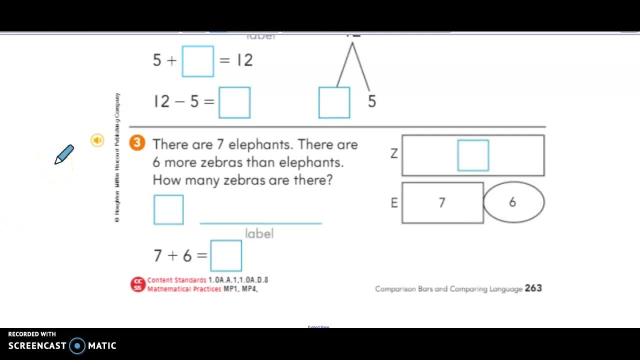 There are seven elephants. There are six more zebras than elephants. How many zebras are there? Okay, so we have the elephants. We label that one on the bottom because they told us that there are more zebras. Okay, so that's why zebras get the top spot. 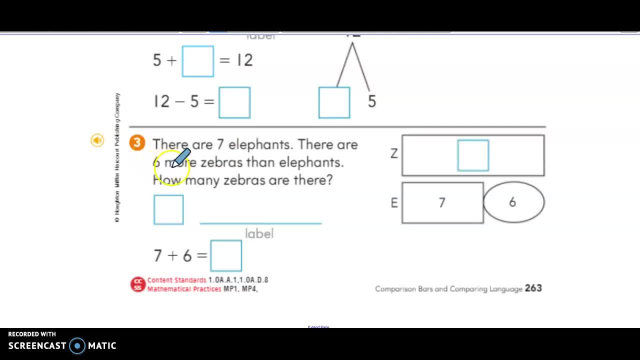 because there's more of them. And then it told us that there are six more zebras, so that's going to go in the oval because it said more- That's a special word, So we're looking for how many zebras, So we don't know the number that's going to go out here. 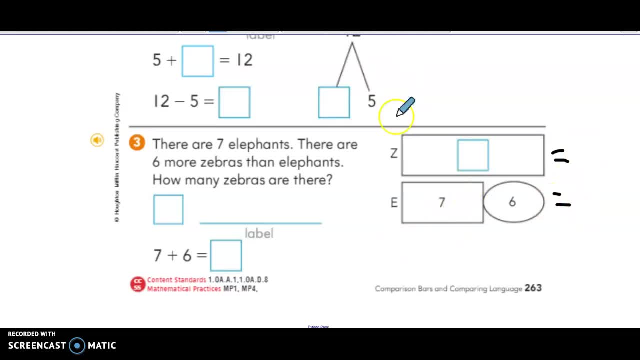 Okay, I can also see here that we would be looking for the total. Okay, just like we can pretend, like this is our math mountain, We can see right here seven plus six. Okay, so grab the seven in your hand and go up six. 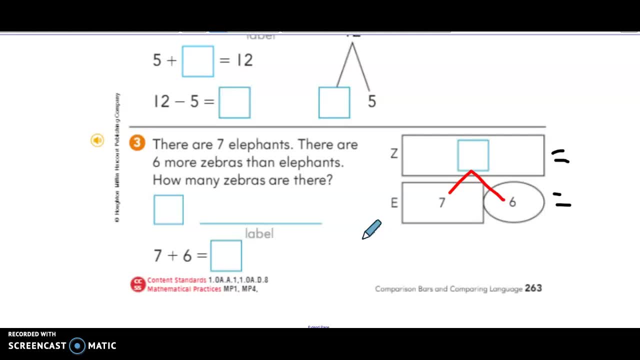 What do you land on? You might actually be getting to the point where you're starting to get a little bit more zebras, So we're going to have some of these facts memorized, so that might make your life a little bit easier. 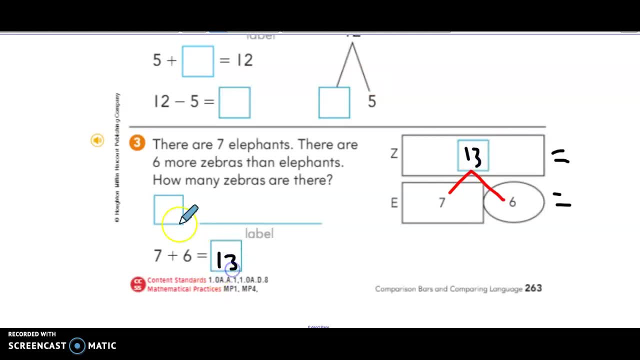 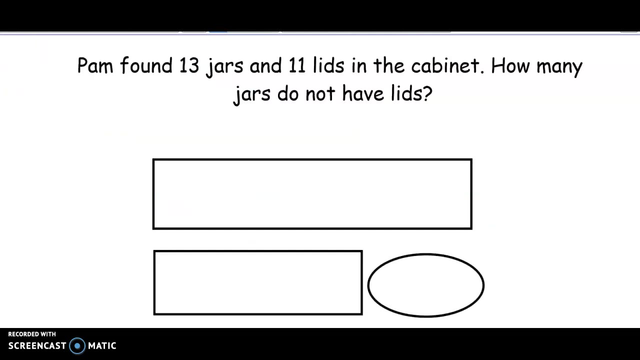 All right, so the number that goes in that unknown box is going to fill up all the unknown boxes, right? And let's check the question for our label: how many zebras, Zebras? Okay, good, Okay, good. Now here is a comparison bar problem. 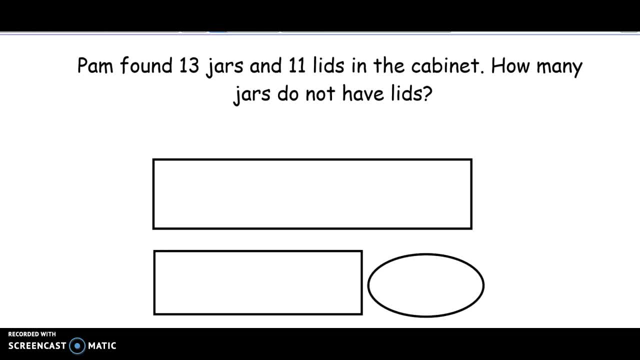 Okay is a little bit different, So listen carefully. It says: Pam found 13 jars and 11 lids in the cabinet. How many jars do not have lids, Okay? so the first question we're going to ask is which: are there more of jars or lids? 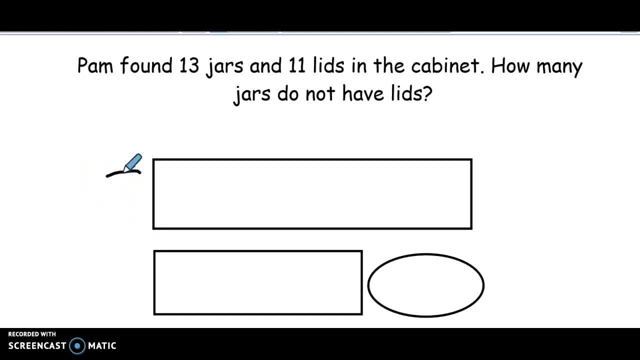 Yep, there's more jars. So we're going to label the J on top for jars, L on the bottom for lids, and let's think about what information we know. Okay, how many jars are there? 13. Okay, we're going to put that out to the side right away. 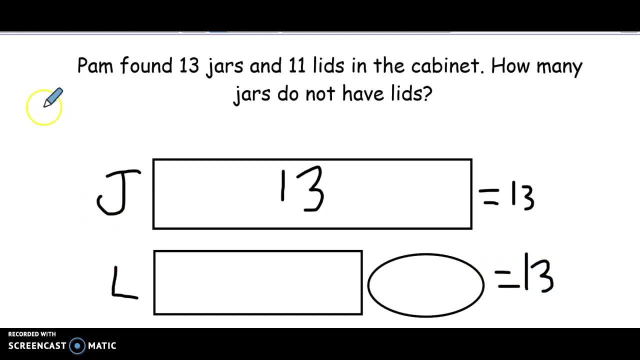 Okay, I noticed that there are. there's no language saying more or fewer, So we have to take the information that we do know and try to figure it out. We have 11 lids, So here's lids: We have 11.. Okay, we just have to think about how many are missing, Like what's not going to. 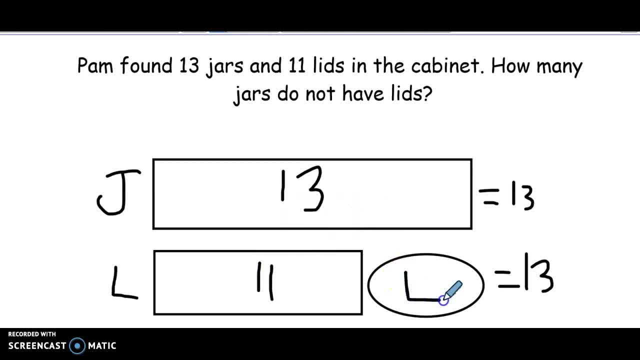 match up with jars and lids. So that's going to be right here in our oval. That would be the difference of what does not match. Okay, so we have 13 is kind of like our total. if we're pretending this is a mountain Or if we have an equation, it would be 11 plus what gets us to 13.. 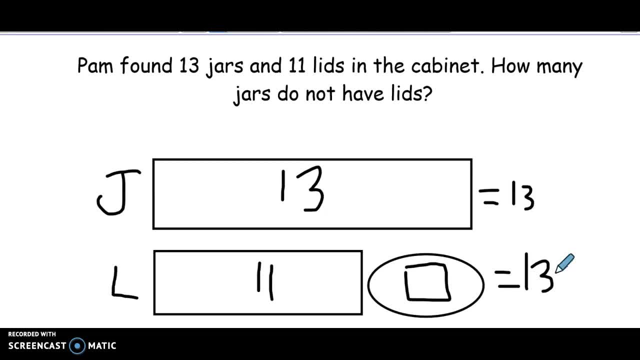 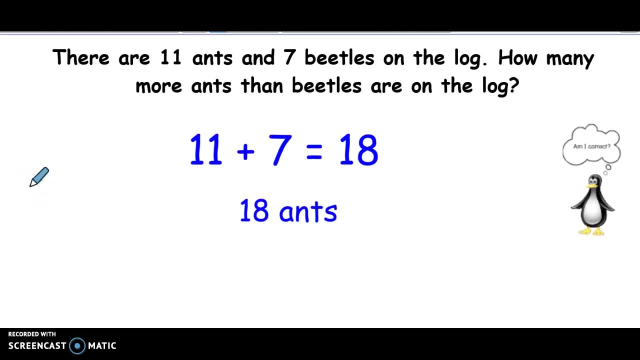 Okay, so grab the 11 in your hand. 11,, 12, 13.. Check your fingers: Yep, it's two. So two jars do not have lids. Good work, All right. so Puzzle Penguin is having an issue here. It says there are 11 ants. 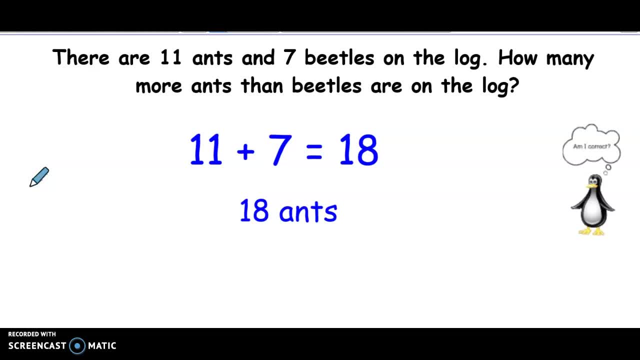 and seven beetles on a log. How many more ants than beetles are on the log? So Puzzle Penguin took these two numbers, added them together and said, yep, it's 18.. Okay, what do you guys think? So we have 11 ants. We're probably going to need to draw some comparison bars here. So this is. 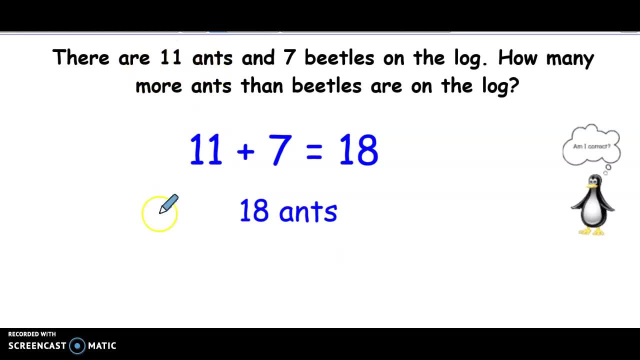 going to give us an introduction to the backside of our worksheet. Okay, and there are seven beetles. So which one is more? Yep, there's more ants, So you can just watch me draw these ugly things. for right now, Ants go on the top and there's 11 of them. Okay, beetles go on the bottom. 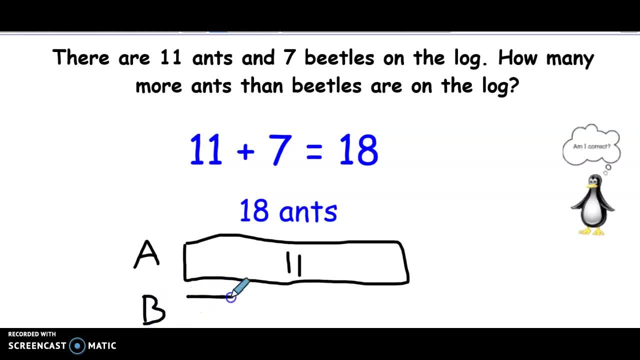 and there's seven of them, So I'm going to draw another rectangle. Okay, they told us that there are seven beetles. Now we need to know how many more ants than beetles there are. So that's going to be our difference, right here, Okay, and 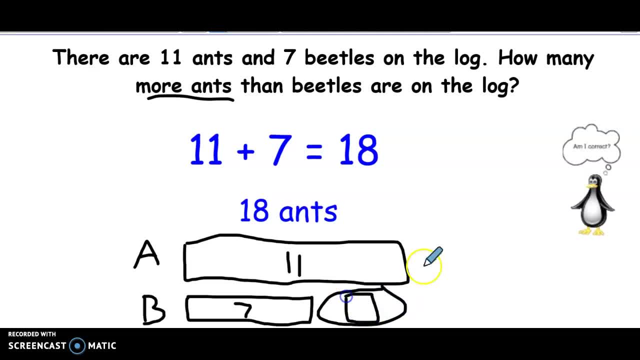 we're going to put our unknown right inside. Out to the side, we're going to put our 11.. 11 is the most that there can be, right, That's, it cannot be more than 11.. So we're going to put our 11.. 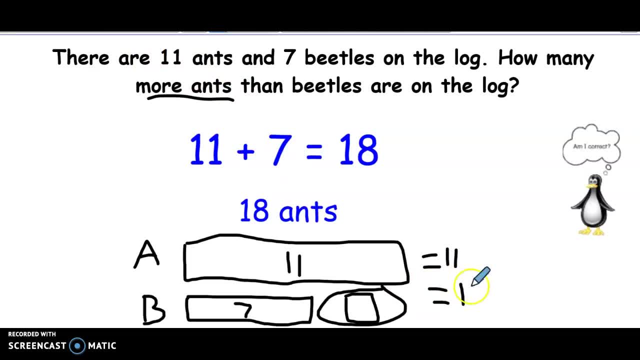 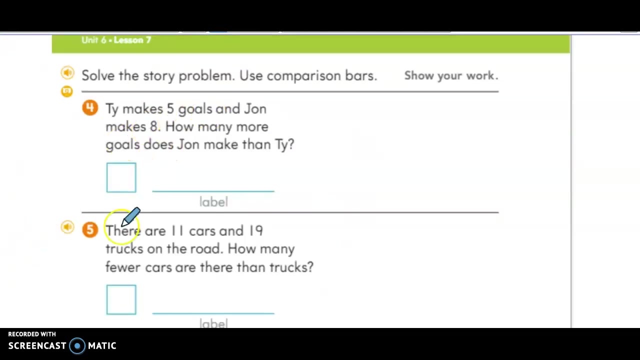 Okay, so this equation that Puzzle Pingo came up with is not correct. We have seven plus what will get us to 11?? Yep, it's four. Good, So our answer would be four more ants. All right, let's go to our workbook, the backside of the workbook page. All right, due to the time constraints. 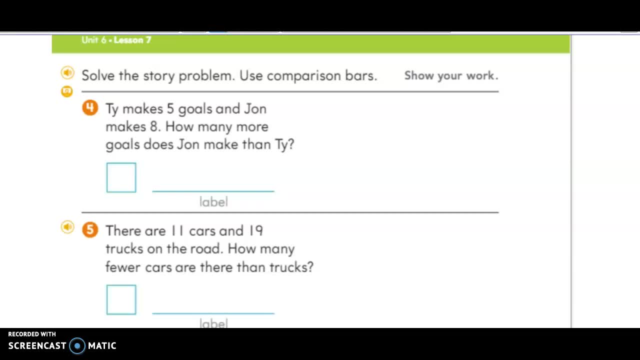 on the videos that I make. I can only talk for about 15 minutes, So I'm going to show you how to set these up, And then I will pause the video And you guys can continue to work. Then, when you play the video, I will have the answers on the screen. So I want you to try them on your 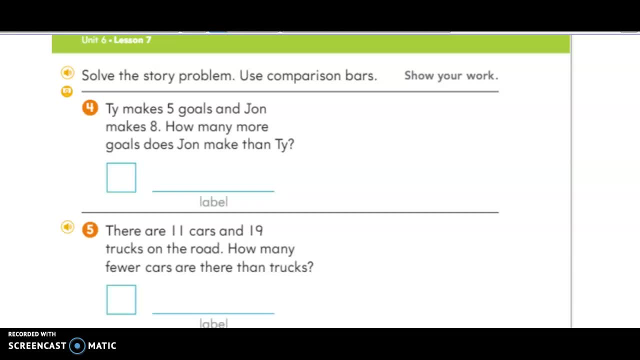 own first, And then, if you get stuck, you can look and see how it's done. Okay, so let's try this first one. Ty makes five goals and John makes eight. How many more goals does John make than Ty? So who makes the most? Okay, John makes eight, So that's more. We're going to put a J for John. 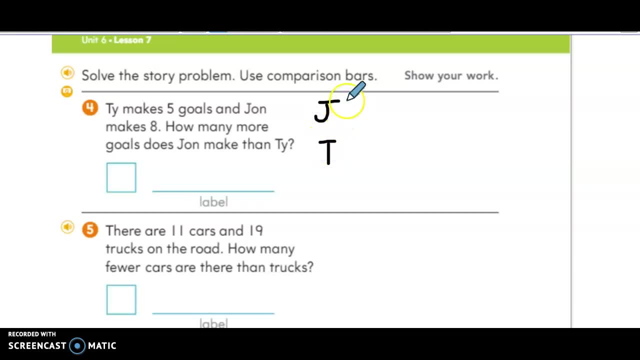 And underneath we're going to put a T for Ty. Okay, we're going to make a bar Now, hopefully your bars are more beautiful than mine. Okay, John made eight. Put an eight up here. Okay, Ty makes five. And then we have our oval. Okay, we only want the oval to be as long as this one. It's kind. 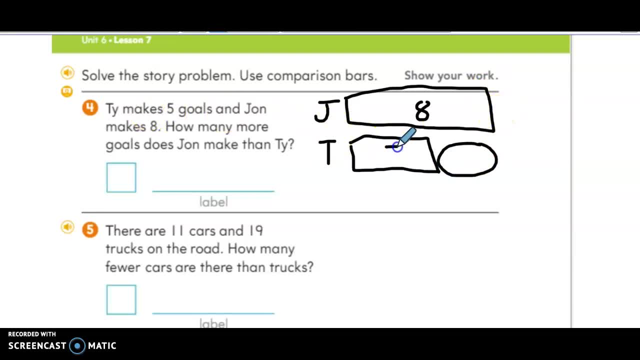 of got to match up. Okay, and we know that Ty makes five, So let's put five here. Okay, we're looking for how many more goals John makes than Ty. More is our special word for the oval. That's the difference. That's what we're looking for. We're going to put our eight out here. 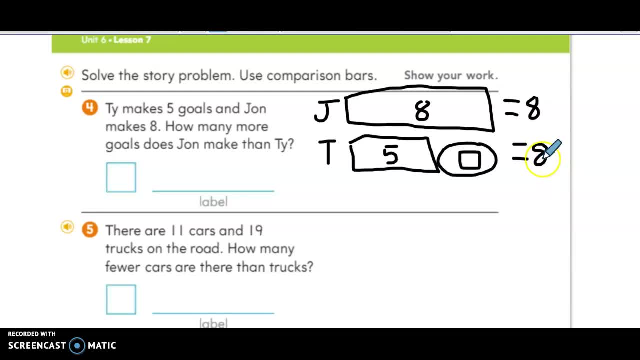 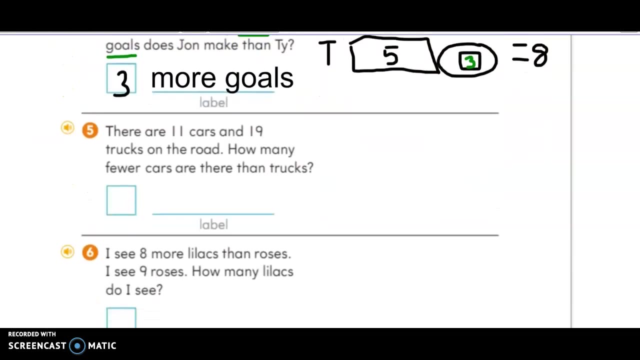 Good, So this ends up being five plus what will get us eight? That's going to be our answer, Okay. Okay, did you come up with three? Great job, So three, and we check the question. more goals. Number five says there are 11 cars and 19 trucks on the road. How many fewer cars are there than 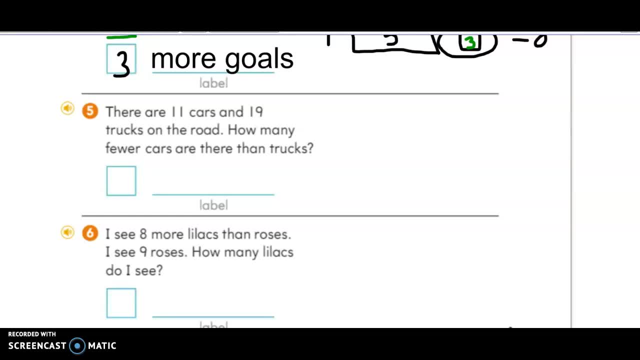 trucks. Okay, so here we go again. Let's ask ourselves who has more. I mean, what is there more of? Yep, there's more trucks. So let's label with a T for trucks, a C for cars. And there's 19 trucks, So we're going to make a big. 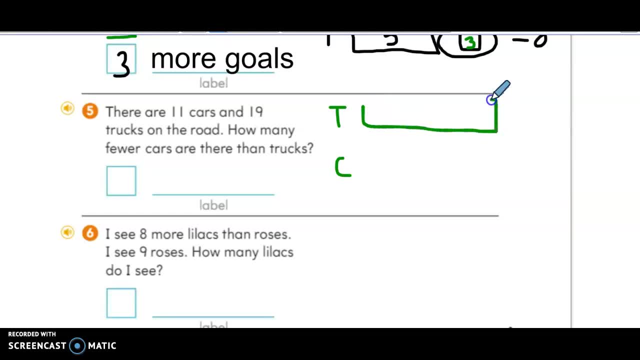 long bar here And it's very important that you are also doing the comparison bars. So draw these out: 19 trucks, Okay, 11 cars. Sometimes I try to guess to see. Hmm, How long should I make this second one, So that it kind of makes sense: 11 cars, Let's put that in. 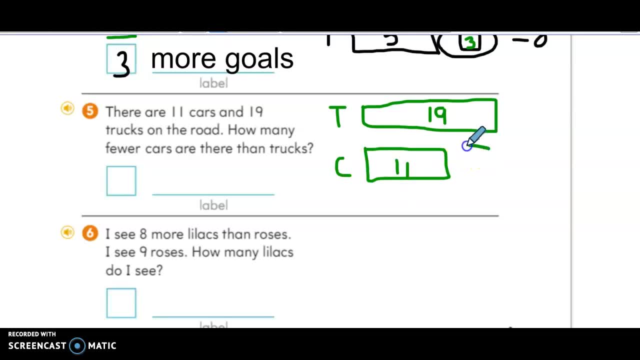 We're looking for fewer cars, So we're going to make our oval. Okay, put your equals 19 out to each side. Good, So this is your unknown 11 plus what We'll get you to 19.. Remember, you can think of this as a mountain. Go ahead and see if you can. 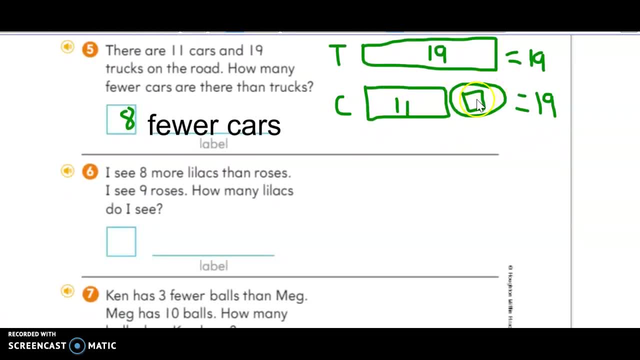 figure it out. All right, I got eight fewer cars. Eight goes here, Eight goes here And fewer cars is in your question. So that's your label. Number six says I see eight more lilacs than roses. I see nine roses. How many lilacs do I see? So you have to think: what do we see more of? 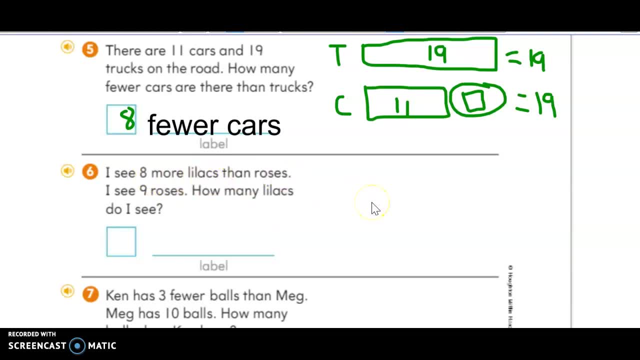 Right, Right. here it says eight more lilacs. Okay, So we need to set up our comparison bars So we see the most of lilacs, right? So we're going to make an L for lilacs. We're going to make our big long bar on the top. Remember the long. one's always going to go up there. 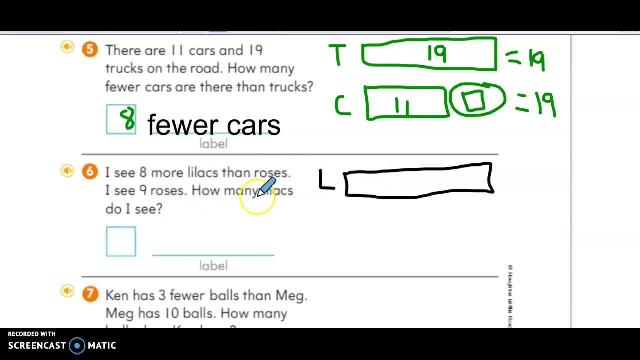 Okay, but we don't necessarily know how many lilacs, because that's what our question asks us: How many lilacs? Well, we don't know right now. Okay, we're going to put an R on the bottom for roses. Okay, roses and our oval: Okay, we know that. we see nine roses, So that can go here.